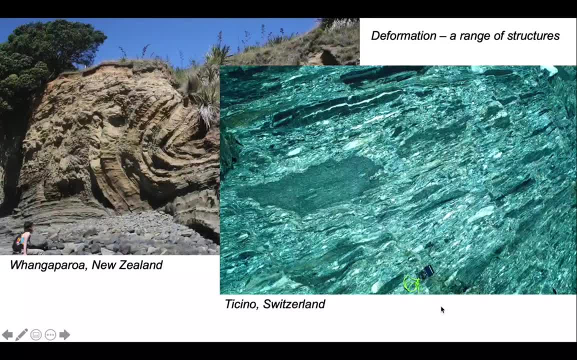 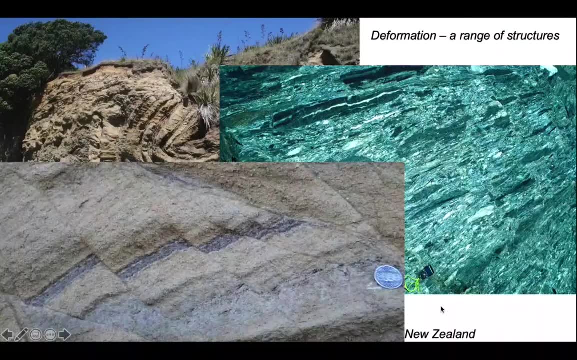 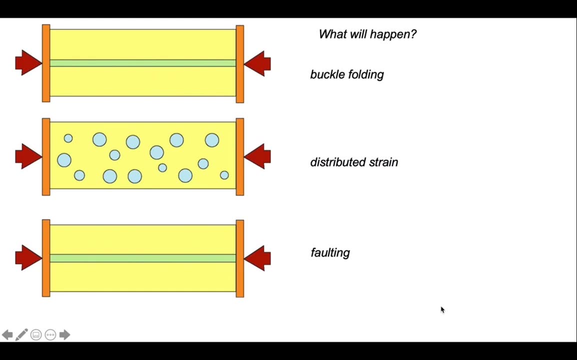 strongly elongated, They look streaked out. And here we are back in New Zealand. This silty layer in sandstones is offset, It's faulted. So let's explore how these structures might develop. We're going to do this in an animated experiment and we'll squeeze these. 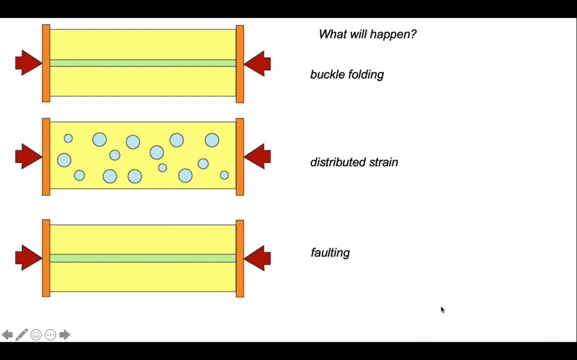 features in a rig. So let's explore how these structures might develop. So we're starting off with an unsqueezed layer And we're going to do this in a swash, undeformed state, And each of these three will deform. 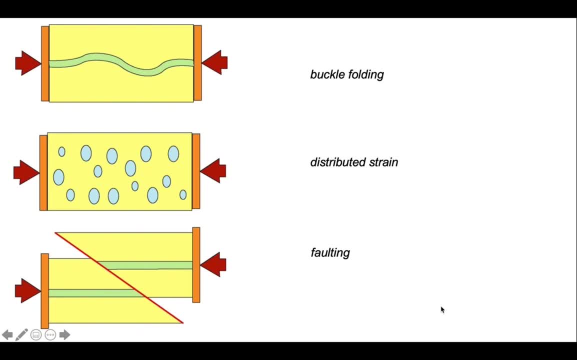 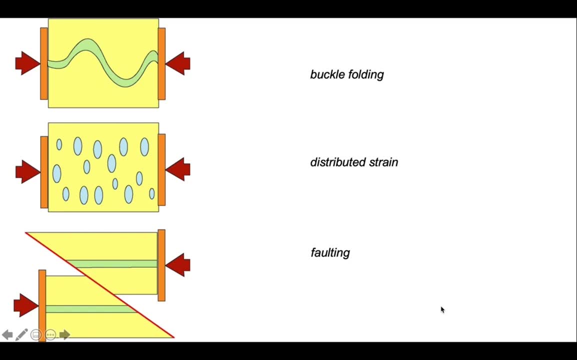 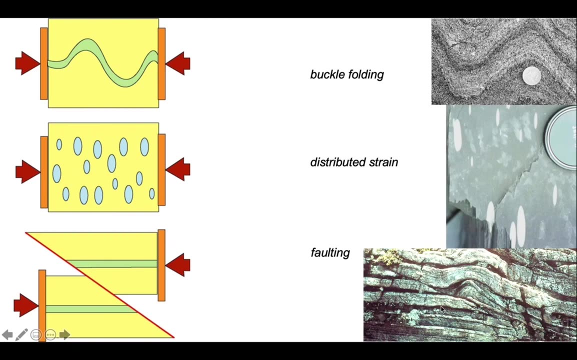 in a different way And we can see counterparts to the structures that we've created in nature. So at the top we can see a fold structure, a buckle fold. So those pale elliptical patches in the slate in the middle photograph were once believed to be circular and preserved. 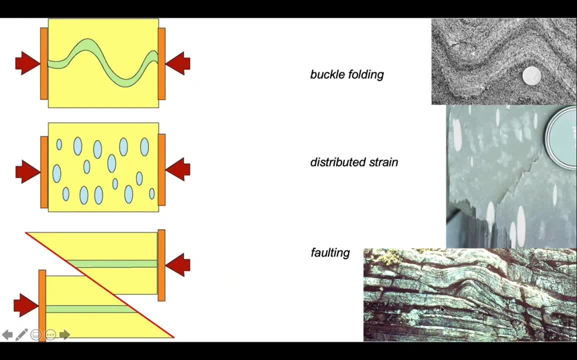 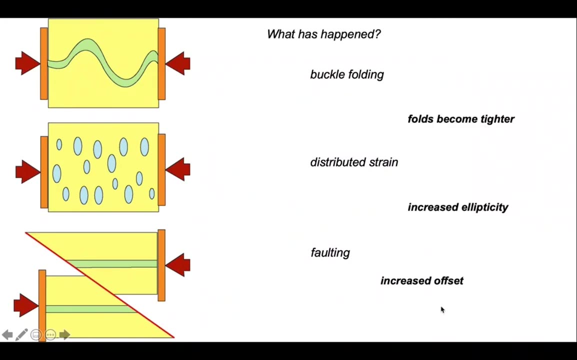 in shape. Presumably, therefore, they've been distorted into the elliptical shapes we see today, And in the lower photograph we can see a fault running diagonally across those gneisses. So we can ask: how did we make the final structures? What's happened? 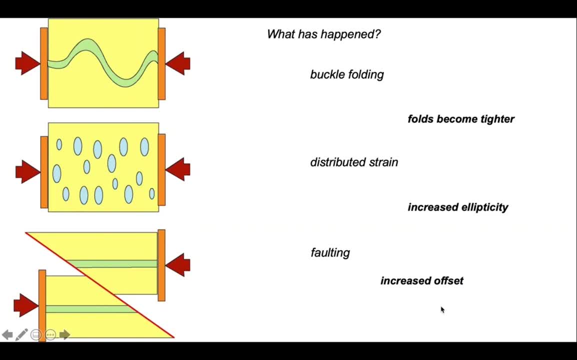 Well, during the progressive deformation for the folds, the folds became tighter. In the middle diagram the region in the vice became distorted through distortion And the distributed strain and the ellipticity of our markers increased. And in the lower diagram the fault increased in offset the more squashed the model became. So these are different types. 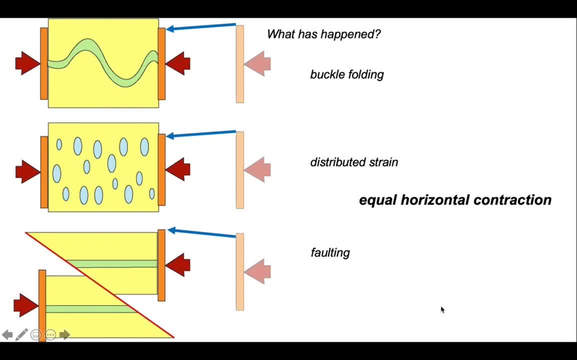 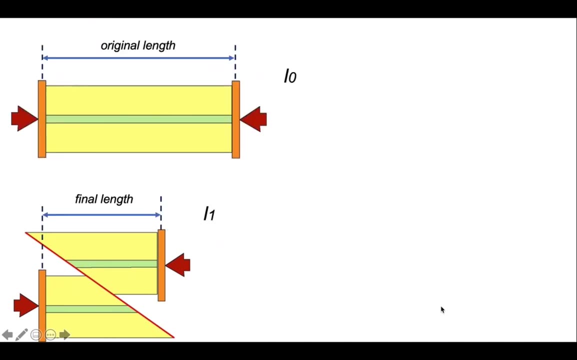 of structures, but they all formed with the same amount of deformation and equal horizontal contraction. in our little experiments, Let's look at the bottom diagram and quantify the amount of contraction. We can do this. This is simply the difference between the original length, which we can. 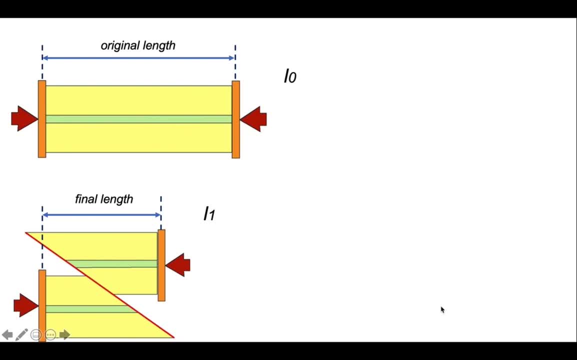 call L0, and the final length of the model, which is L1.. This comparison in structural geology is called the longitudinal strain E, which stands for elongation, And it's simply the difference between the original length and the final length divided by the original. 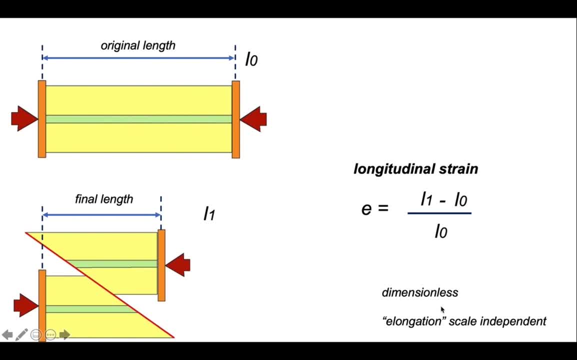 length. Both top and bottom of this relationship are the same length. The elongation is dimensionless, so it becomes a useful parameter because it's scale-independent. Let's have a brief aside and look at what happens if our model is pulled apart, not 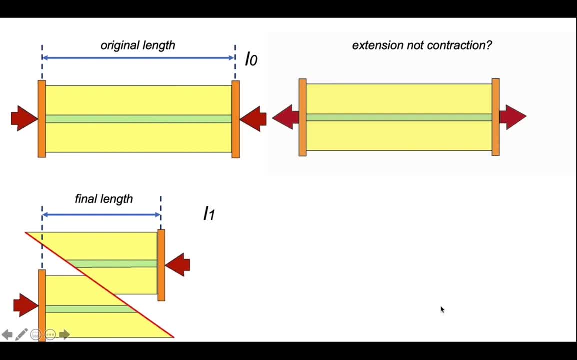 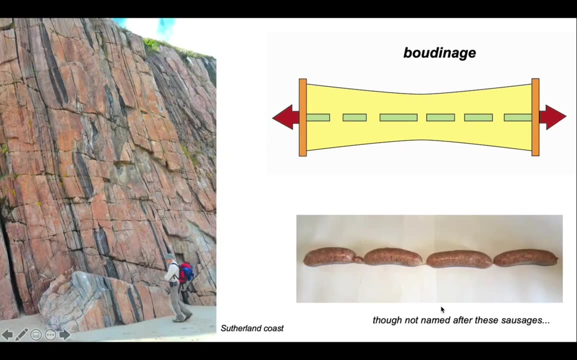 squashed together. So we're dealing with extension, not contraction. Well, the green layer is going to be pulled apart like this. This type of deformation is called boudinage, named after the French for a type of sausage, And here on the outcrop we can see a natural example with that black amphibolite layer. 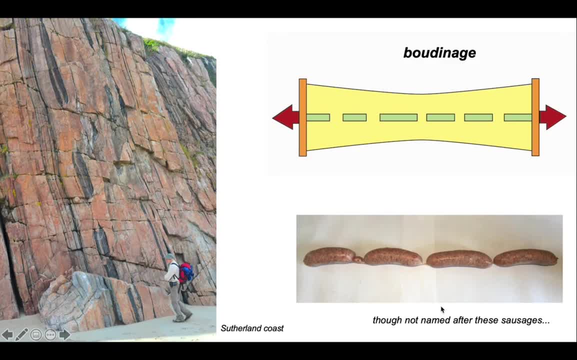 we assume was originally continuous and we infer therefore that it's been pulled apart, as these rocks, in their present orientation, have been stretched up and down the length of the outcrop. So here are the boudins, The sausage is on the outcrop. 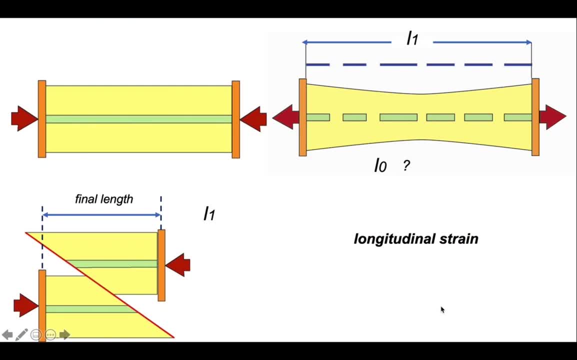 As with the contractional case, we can quantify the longitudinal strain for the boudinage situation. L1 is simply the modern length between two known points along our string of sausages. But what is the original length? Well, that's simply the sum of all the various lengths of individual boudins, of the individual 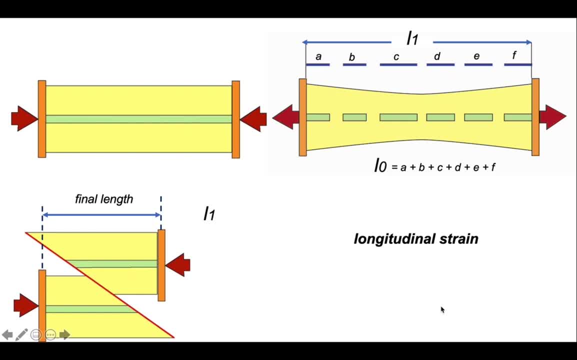 sausages. So add them together and that is the original length. Assuming that they have not become the same length, we can simply add them together And we can plug L1 and L0 into the expression for longitudinal strain. Notice, we can do the same thing for the contractional faulted case on the left-hand side, because 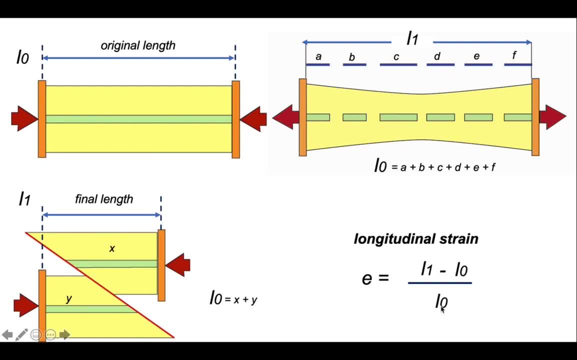 we don't get to see the original geometry, But from the final state we can use those two segments of the green layer, x and y, and add those together to find L0. So the parameter L0 is the original length And we can plug L1 and L0 into the expression for longitudinal strain. 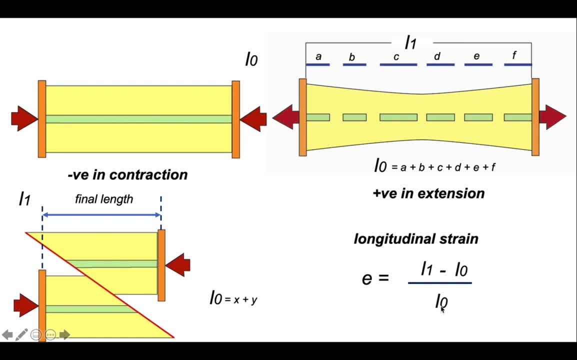 So the parameter e, elongation, is a positive value in extension but a negative value in contraction, because in extension L0 is shorter than L1. So the expression on top of the equation is positive, whereas in contraction the final length is shorter than the original length, therefore the top term in that expression 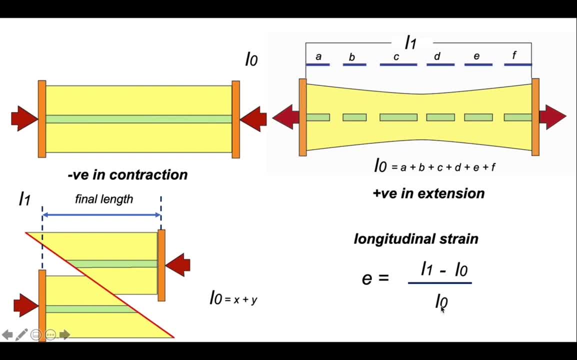 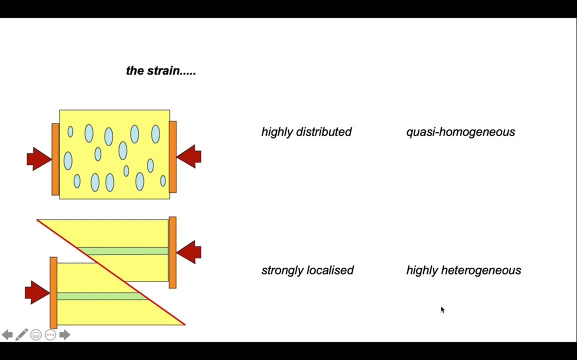 is negative, negative, the whole expression becomes negative. So let's move back and look at the distorted version. We can think of this in terms of the localisation of deformation. In the lower faulted example, all the deformation localised onto an infinitesimally narrow surface. the 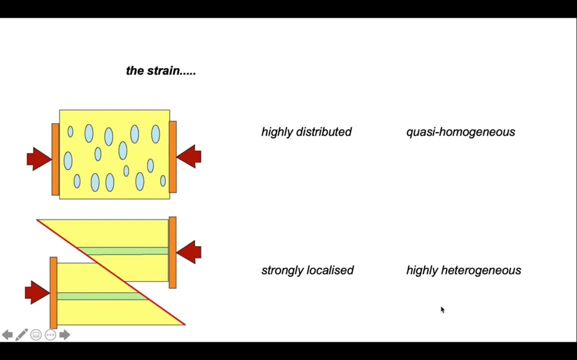 fault plane. In the version on top, the deformation is dispersed through the entire volume and is therefore highly distributed. You may think of the strain in that upper case as quasi-homogeneous, but in the lower one as highly heterogeneous. This allows us to make a point, because it's 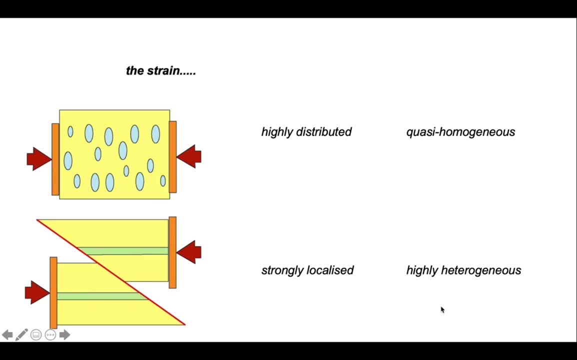 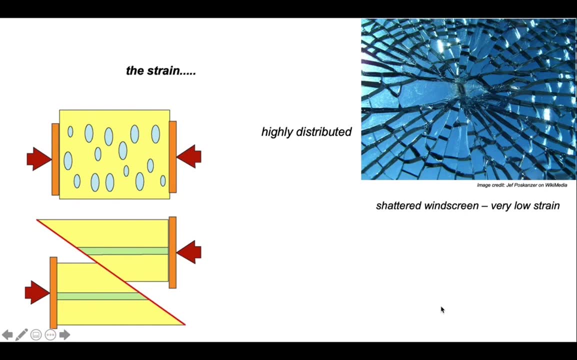 tempting to suggest if deformation is highly distributed it is also a high strain. Well, consider a shattered windscreen in a car. There are fractures all the way through it. so there's a highly distributed, dispersed fracture, But the windscreen itself can retain its original shape, so has a very low strain. there's. 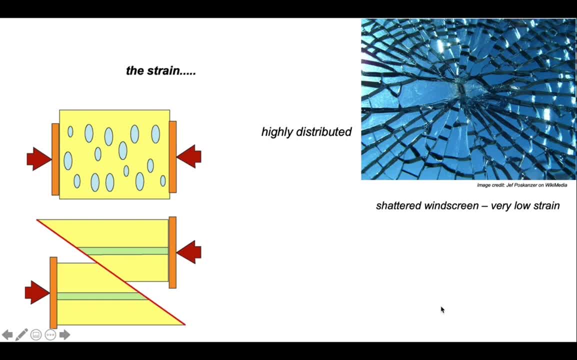 a very low distortion to the windscreen even though it's highly shattered. So the distribution of deformation is not a proxy for the strain state. That point made, let's go and have a look at this distortion So we can see as a consequence. 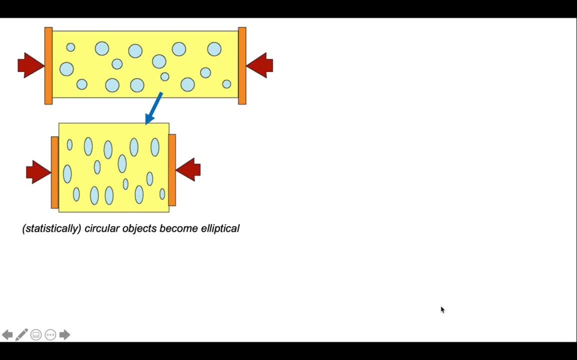 of squashing our model together, that our originally circular objects have become more or less elliptical. This allows us to introduce the concept of the two-dimensional strain ellipse. Before deformation, consider a circle, So this has a single value for a diameter. but if we distort that model, we create an elliptical shape which has both a long and 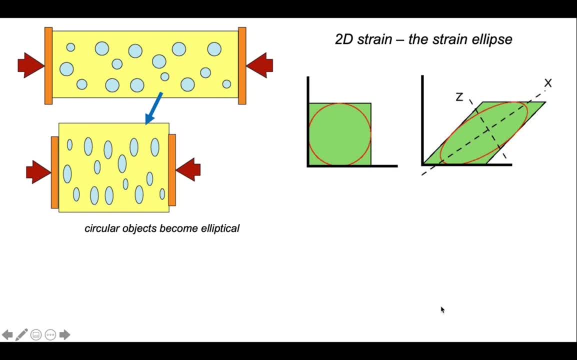 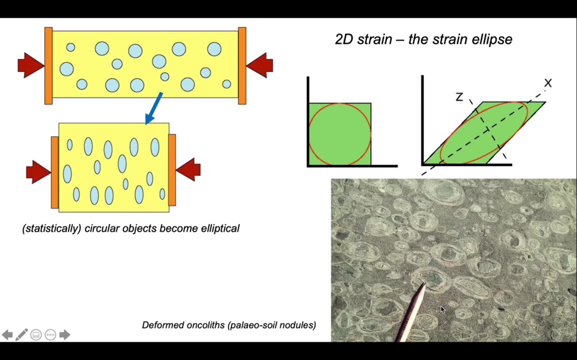 a short axis, So we can quantify the strain through the ratio between the long axis x and the short axis z. Here's an example of some markers that we assume were originally circular in view and they're now elliptical, So we measure the shapes of these features. we can quantify.